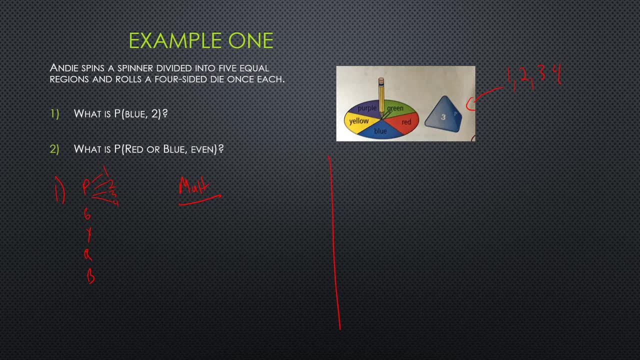 So the answer is one, When we look at our spinner. we're going to kind of break it down to two probability questions. So the first part says: what's the probability of getting blue? Well, when we look at here, there's one blue out of how many total? Well, there's five possible outcomes. 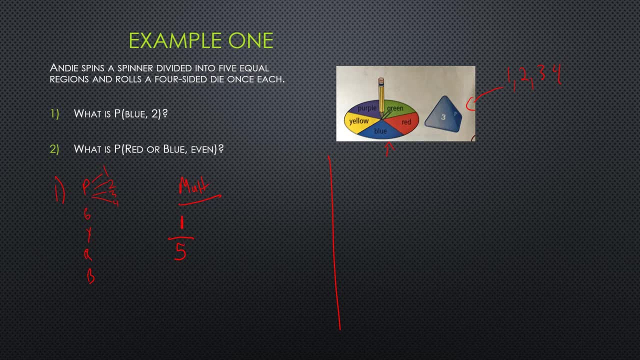 So we have a one out of five chance of getting a blue on the spinner, And we're going to multiply that probability by the next one. We're looking at a two. Well, on that die, there's only one two. So we have one chance of rolling a two on that die And there are four possible outcomes. 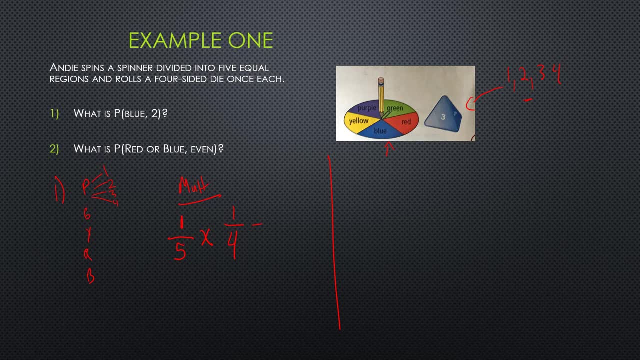 So we multiply our probabilities together. Now that gives us a. one times one is one, and five times four is 20.. That gives us a one in 20 chance of getting blue two. So it just really saves a lot of time, whereas you still could easily do your tree diagram like this, You know. 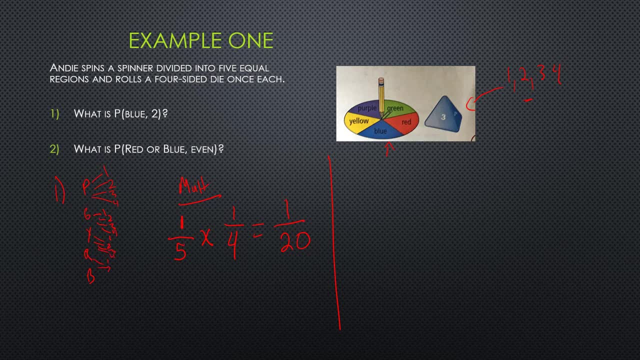 one, two, three, four. one, two, three, four. one two, three, four. And if we look at it right now, on this diagram, blue, two, while blue is right here and there's only one, two. so we'd have a one. And if we count, 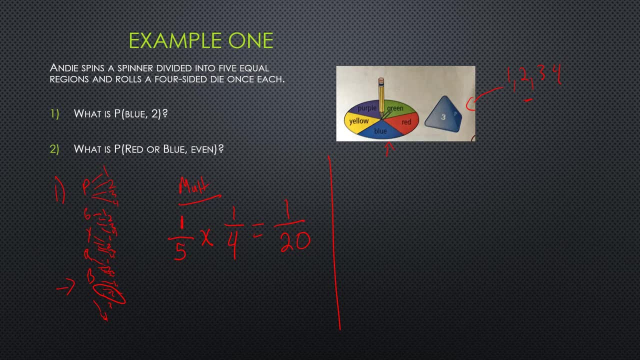 them all together: one, two, three, four, five, six, seven, eight, all the way up to the top, it would still be one out of 20.. So if that works best for you, you can definitely do that. But if 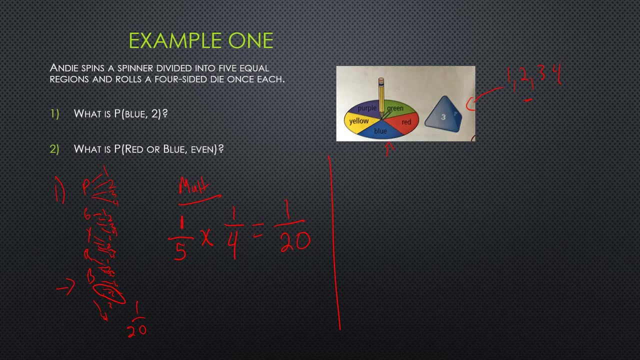 you're looking to kind of speed things up a little bit, you can actually use the other method, which is our multiplication method. So let's look at our second example here. What is the probability of getting red or blue and even Well, again, we've got to do our probabilities of each event here. So what is the probability of? 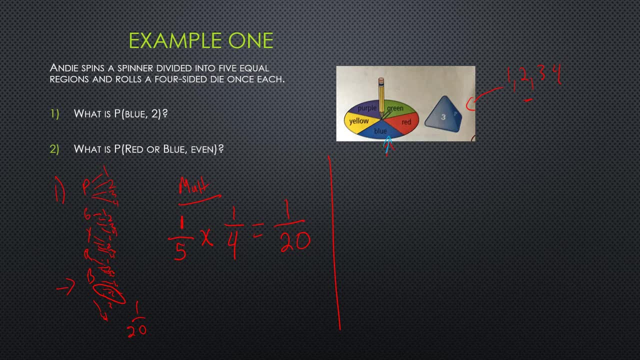 getting red or blue. Well, we have red and blue here. Well, there's two of those out of five possible options being yellow, purple, green, red and blue. So we have two, because red or blue is two of the options, And we're going to multiply that probability by even. Well, on the die. 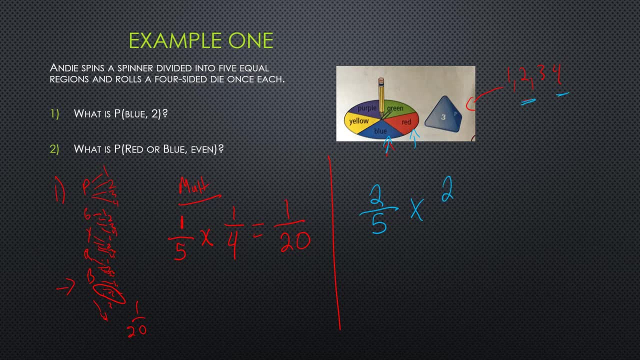 we have a two and a four, So there are two possible even numbers and still four total numbers. on that die one, two, three and four. If we were to multiply this together two times two is four And we're going to find: 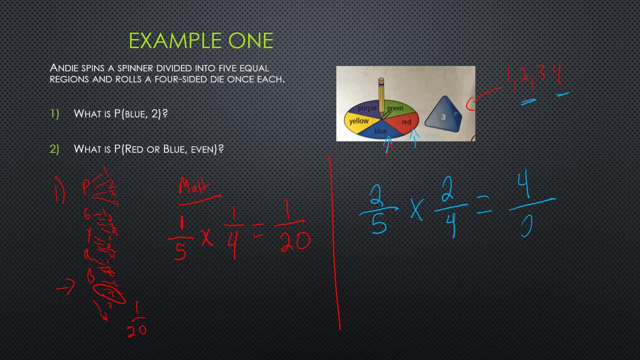 that four times five is 20.. So we have a four out of 20 probability of getting that answer. If we were to narrow that down even more, we can divide four by itself and 20 by four, and we would get a one. 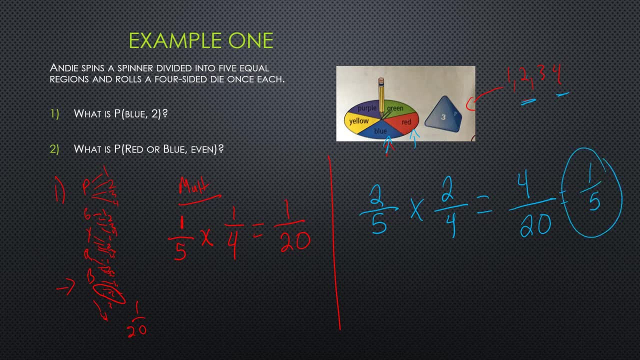 So we would get a one in five chance. So our probability of getting is one in five if we're looking just for a fraction. So that's how you can use multiplication to solve your answers, And I'll take a look at our next example. 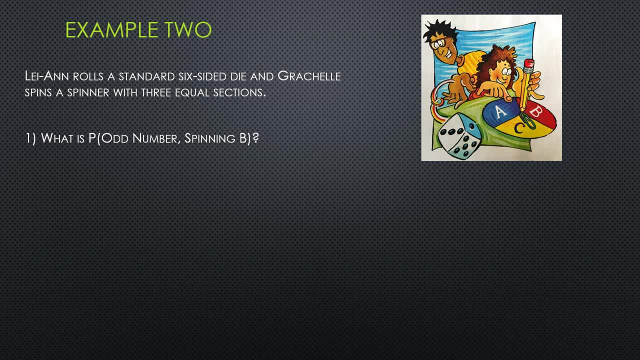 So example two says Leanne rolls a standard six-sided die and Grishel spins a spinner with three equal sections. Now, sorry, the only picture I could find that had something like this does not depict both people in this example, but that's okay. 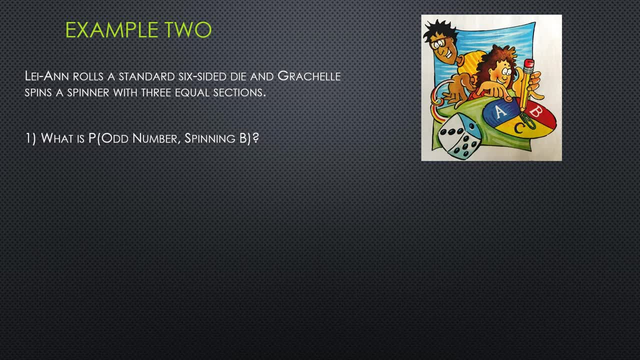 What is the probability of getting an odd number and spinning a bead? Well, again, we could do that tree diagram or a table, But for this lesson I'm going to stick to multiplication. So let's start with the first part: our odd number. Well, we know, on that die the six sides. 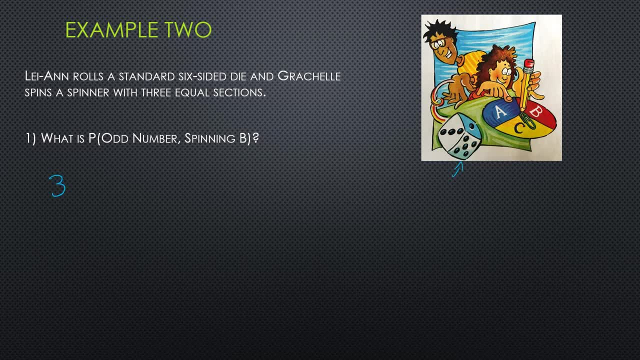 there are going to be three odd numbers possible on a six-sided die. We're going to have one, two, three and five. So our favorable outcome is three. And on that die there are six sides, So there are six possible outcomes on that die. We're going to multiply that probability. 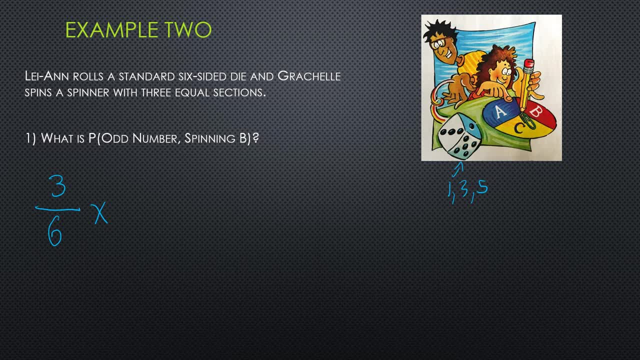 by the next event, which is spinning the three equal section spinner, And it's saying spinning a bead. Well, we can see that there is just one bead there. So our favorable outcome is one And there are total outcomes a, b and c. There are three total outcomes, So we're 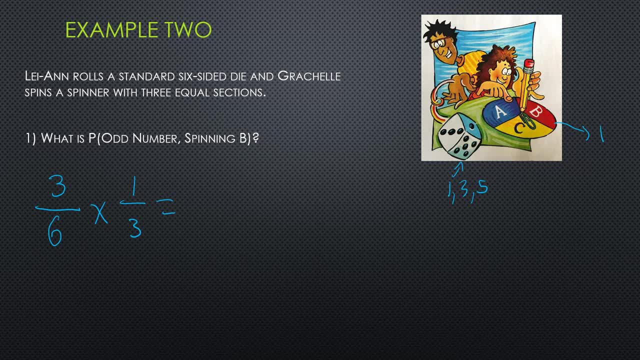 going to multiply this together, We're going to have: three times one is three And six times three is 18, giving us a three of 18 probability of getting an odd number and spinning a bead. However, we can still break this down by dividing the top and the bottom. Three divided by three is one And 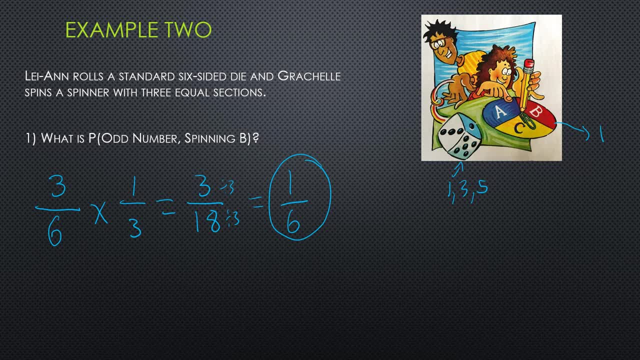 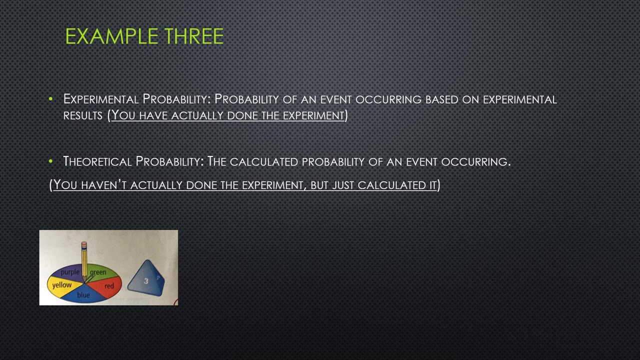 18 divided by three is six. So we have a one in six chance of actually spinning that bead and getting an odd number. So now let's take a look at our third and final example. So example three, First thing we're going to look at here are just two terms, you're. 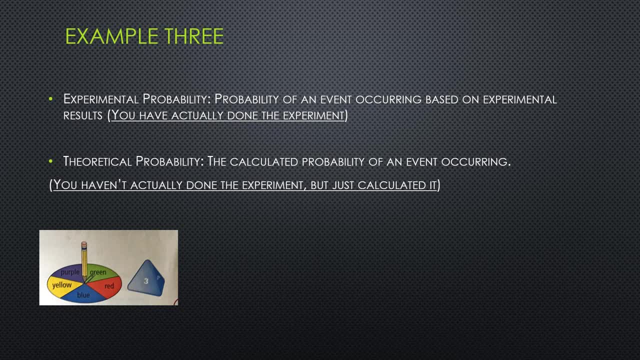 going to notice in your assignments The term experimental probability and theoretical probability. So let's just start with what each one means. So experimental probability: Well, this is the probability of an event occurring based on experimental results. What this means is you've actually done the experiment. So, for example, if it asked like in that first question, 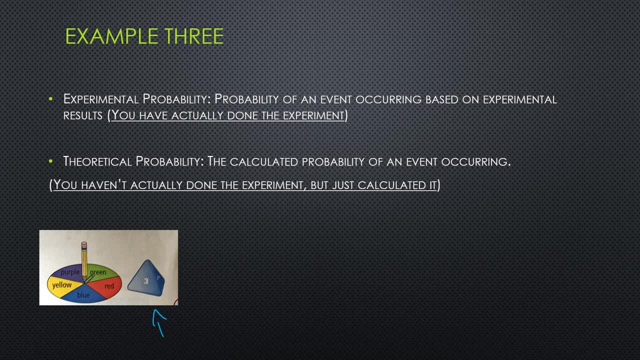 you know your spinning the spinner and rolling the die. it means you yourself actually have a spinner and a die and are actually doing the experiment to see what the outcome is. That means you would actually have been spinning it so many times to see if you were going to get blue. 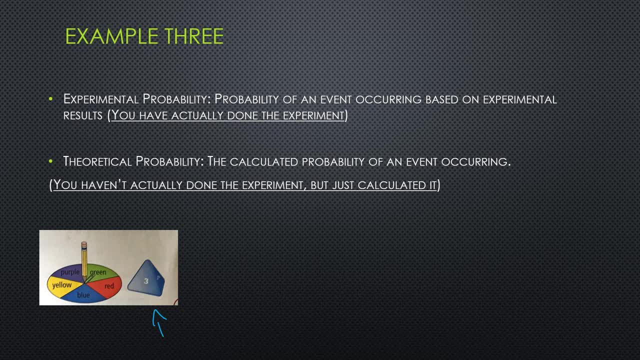 and then a two, And you have tried that multiple times to see if it works. So we haven't done that yet so far because we haven't actually had to do any of the physical problems. But that's what experimental means. It just means you are actually doing it. 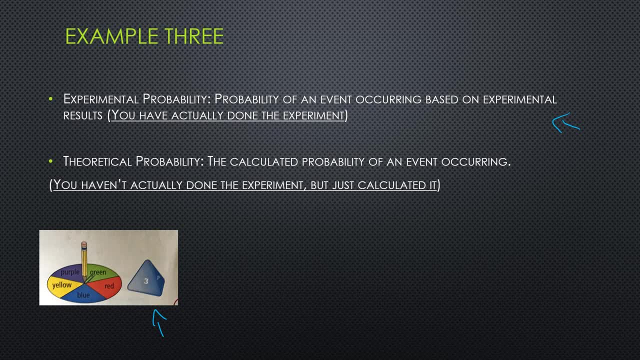 Or theoretical probability. The calculated probability of an event occurring means we haven't done it, but calculate, and that's what we've done so far. We had questions where it said: you know what's the probability of getting blue And a two? Well, we didn't. 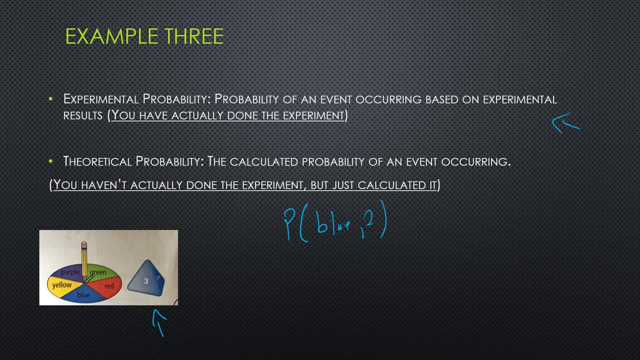 actually in that first example, spin a spinner that went blue and then roll a die. We said, Okay, well, there was one blue option out of five and there is one two out of four. Oh yeah, That gave us a 1 in 20 chance. 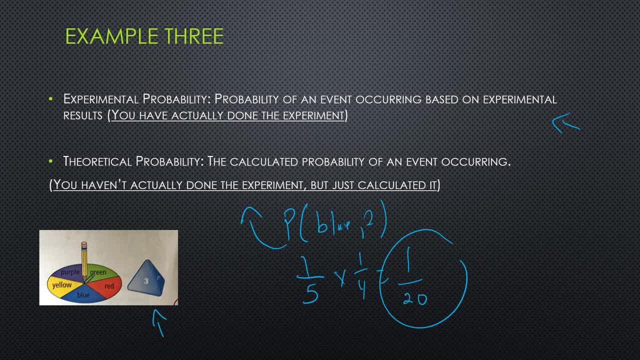 right here is our theoretical, because we're kind of calculating it- what we think it's going to be, but have not verified it by actually doing the experiment. so that's really important to understand the difference between these two. so, with that being said, let's take a look at this question. so example three: 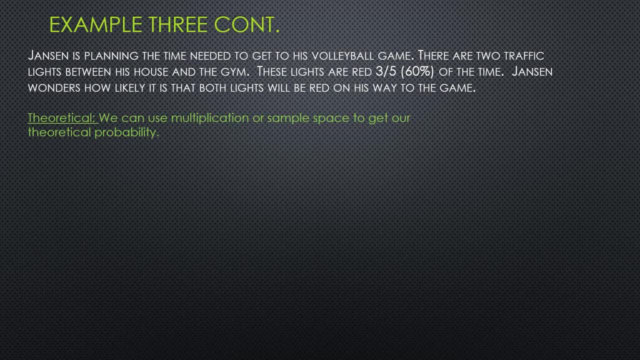 says Jansen is planning the time needed to get to his volleyball game. there are two traffic lights between his house and the gym. these lights are red three, fifths or sixty percent of the time. Jansen wonders how likely is it that both lights be red on his way to the game? so wondering, he's driving in the. 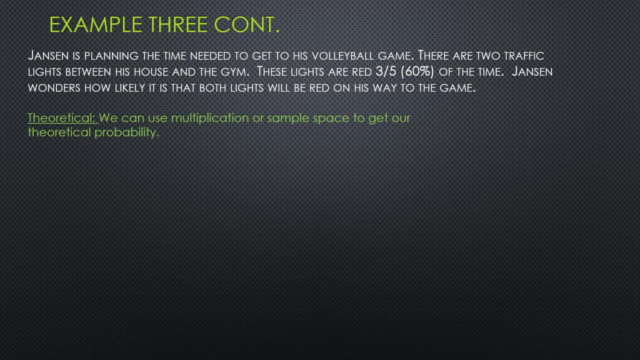 game with his mom. what is the chance that both lights are going to be read, that he hits them well right now, if we're doing this theoretical, we can simply just use multiplication or sample space to get our probability. so let's do that right now. so it's. 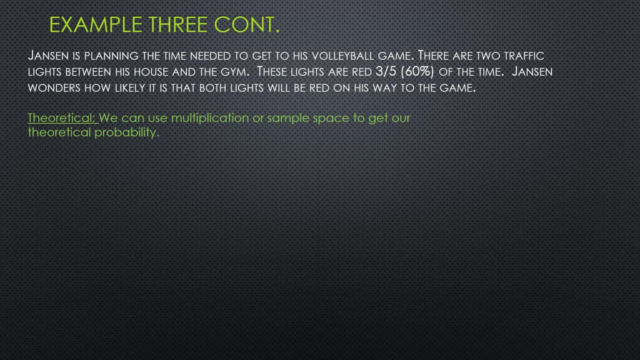 says these lights are going to be read 3, fifth or sixty percent of the time. that means that light one here is going to be read three fifths of the time and light two is also have the probability of being three out of five red. well, the 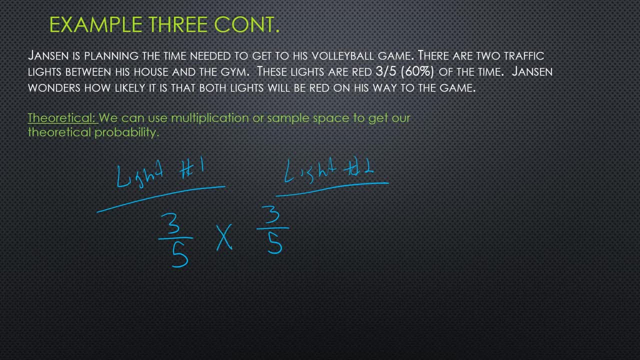 probability of them both being read. we still have to multiply them together. that's our theoretical probability. so three times three is nine and five times 5 is 25.. So we have a 9 in 25 chance of those lights being read at the exact same time. 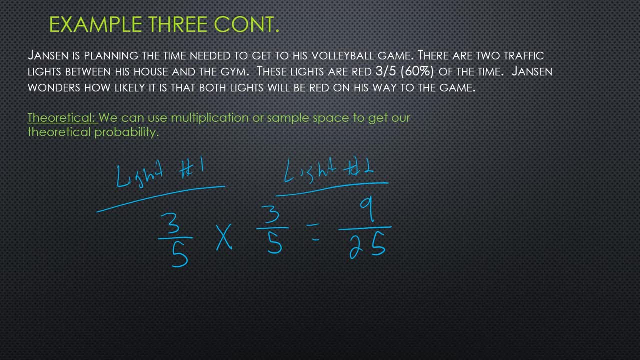 when he hits 1 and then down the tree, the next light. Now, if we were to turn this into our decimal and fraction, if we divided 9, our numerator by denominator, we're going to get a decimal of 0.036 and then a percent of 36 percent. So we theorize, based on that fraction, that those both 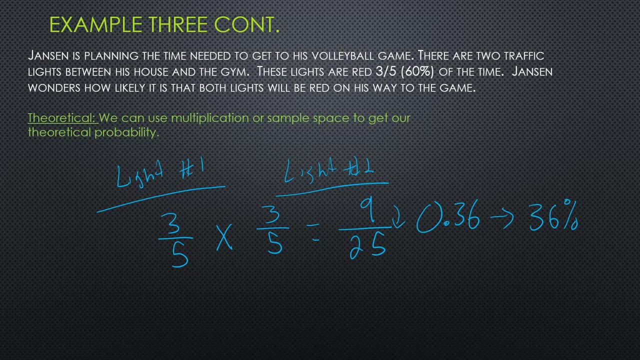 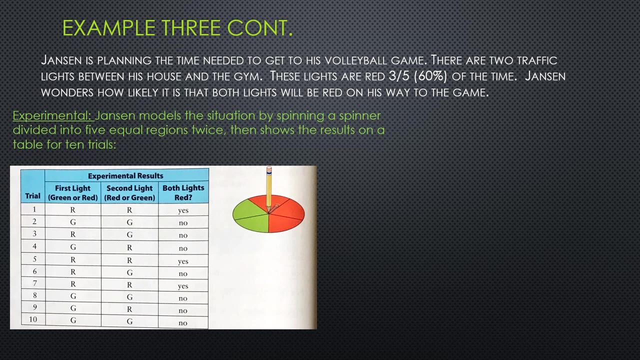 lights he'll hit have a 36 percent chance of being read both times. So that's our theoretical probability. we haven't tried it yet, we've just calculated. Let's take a look at our experimental probability. So same question, but in this situation Jansen wanted to actually test. 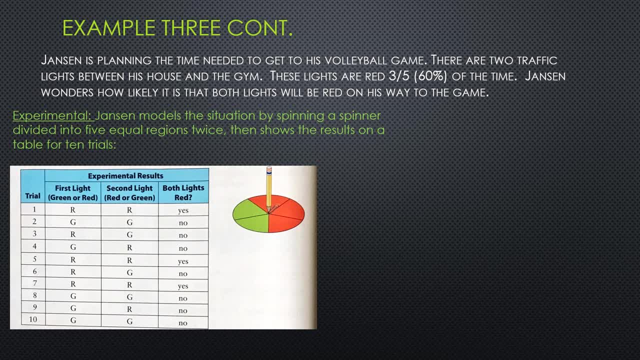 out his theory Now, rather than just drive and hit the lights and just count that each time you went, he created an experiment that he could do that would still symbolize the results of what he was looking for. So what he did is he created a spinner here, as you can see, with three red lights. 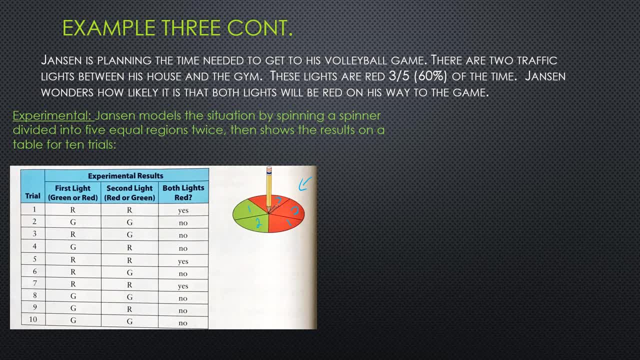 and then two green lights. So the idea here is that if he spins these, you know, twice, first and then second time, and then would double check to see what his results were. So for example, when he spun it the first time he got red and followed by the second time it was red, So both 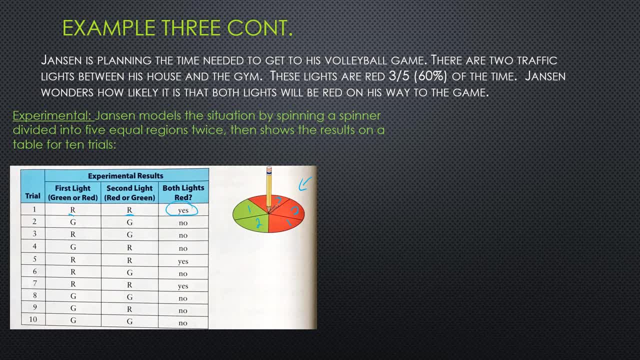 lights were red. yep, that happened. Then he did the second time and it was green and then green. so they both weren't red. And he's done this multiple times to find out, just out of a sample of 10 times, to see what that probability could be. if he tried it out, And he's found here that his 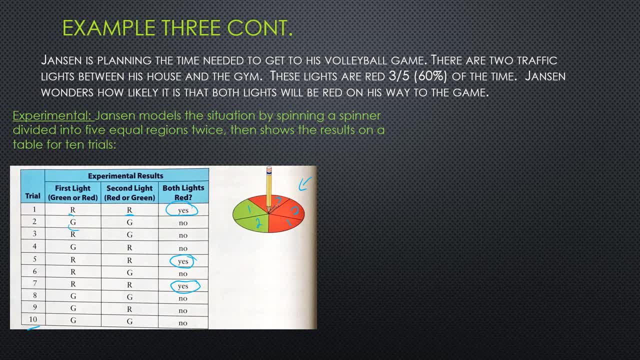 probability here. he did it 10 times. Three of these times both lights were red, like he was looking for. so he found that it was actually a three out of ten chance of those lights being red both times because he's done this experiment. Well, if we make that into our decimal, it's 0.030, and as a percent, 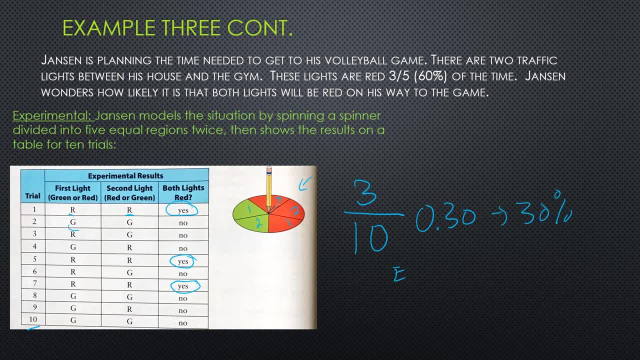 30 percent. Well, our experimental probability was 30 percent, but it differs slightly from our calculated one in theoretical, because we found that it was 36 percent. Now, to be fair, there is what we kind of calculated versus what he actually tried, But he only did it 10 times. The more times 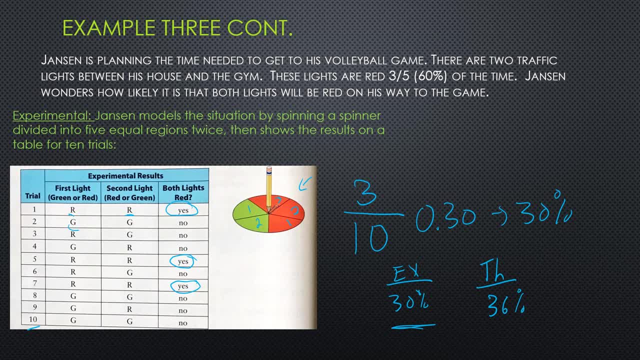 you do a probability experiment, the more accurate results are going to be. So 10 times- yeah, that gave us a good example- 30, and they are pretty close. But if Jansen was to do this, you know, 100 times or thousand times, we might find these two numbers get a little closer. So there will probably 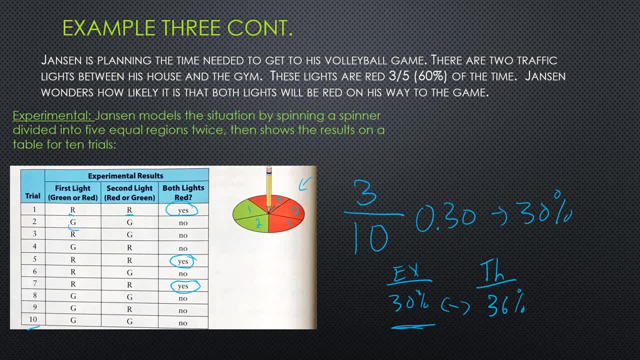 be a difference in our experimental to our theoretical. The more times you do something in something, you do it 10 times. The more times you do it 100 times, The more times you do it in science or math for experiment wise, the more accurate your answers are going to be. So that's. 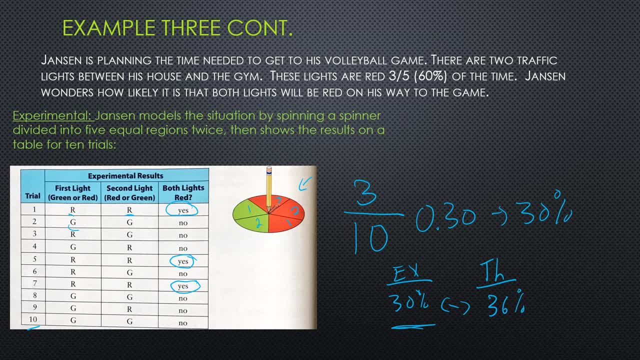 pretty much what you're looking at for today When you get to the questions on your assignments. just remember that experimental- you're actually going to have to design an experiment to check your answers- and theoretical- you're simply just what we've been doing all unit long.